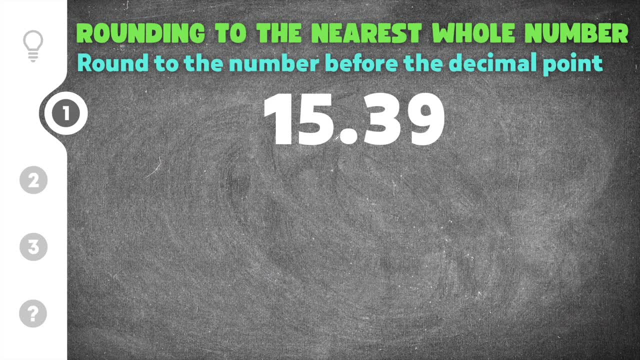 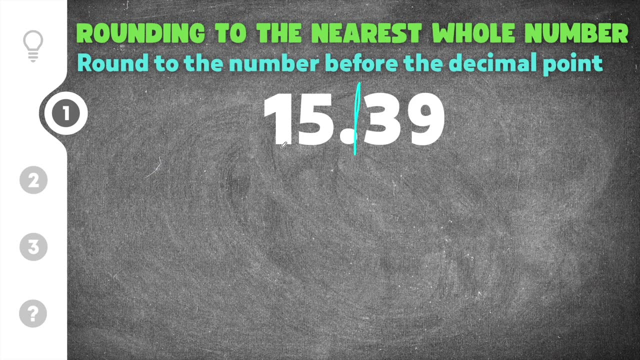 us 15.3.. and asks us to round this decimal to a whole number. So our first step is to draw a line after the decimal, and I know that I'm rounding this 15.. So this 15 is either going to round up to a 16, or it's going to stay a 15.. 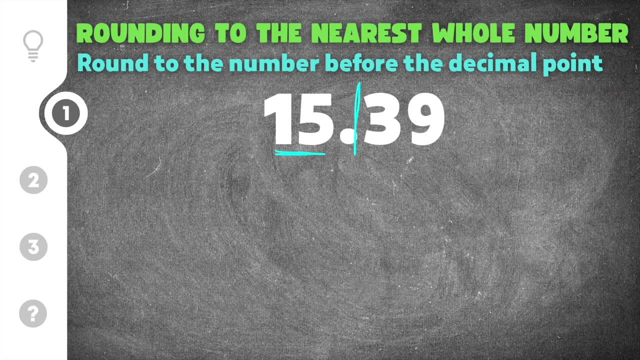 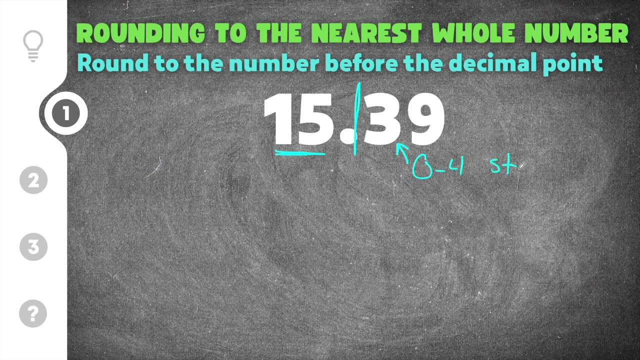 In order to determine that, I'm going to look at the number after my line. In this case, the number is 3.. 3 is in between 0 and 4, which means that our number or our whole number is going. 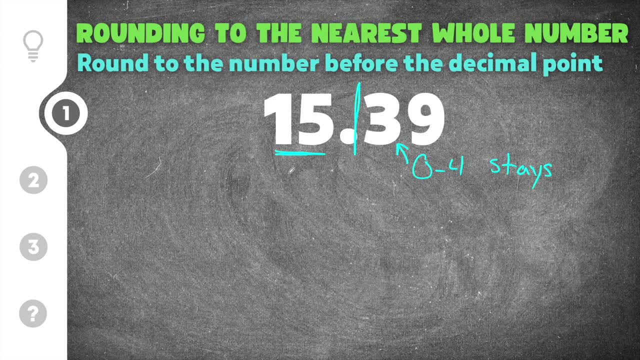 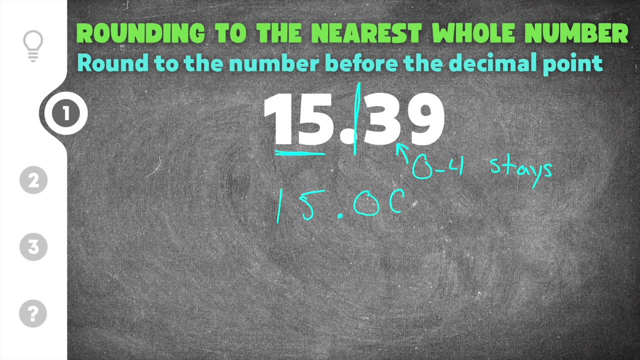 to stay the same. So when I round this, this 3 keeps the 15 just a 15. I'm going to put my decimal point and then everything after that decimal point is going to turn to zeros. So right now I have 15.00. 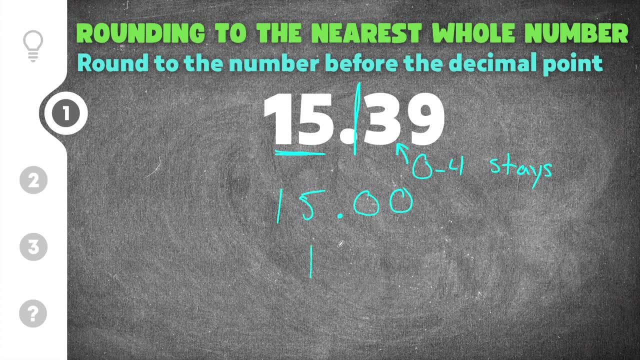 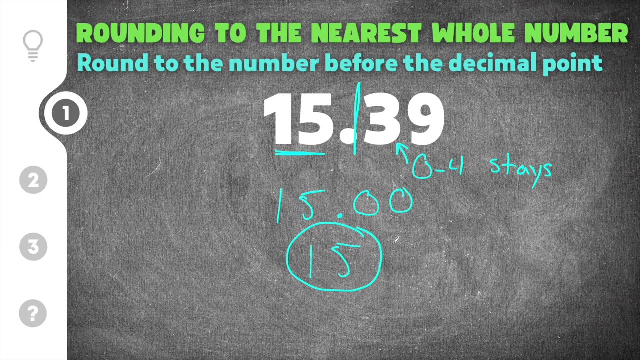 We don't actually need the zeros, because the zeros represent a value of nothing. So 15.39, rounded to this nearest whole number is just going to be a zero. It's going to be 15, and that's going to be our solution. 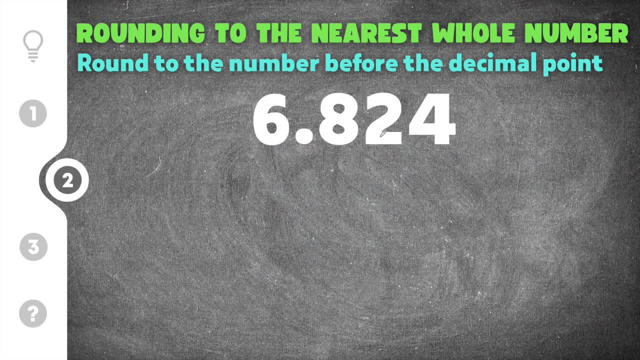 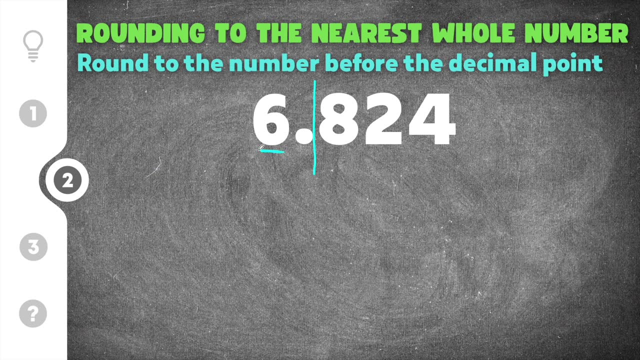 Moving on to number 2.. Number 2 gives us 6.824.. Now the first step for rounding this decimal to a whole number is to draw my line. I know that the 6 is going to get rounded either up to a 7, or it's going to stay the. 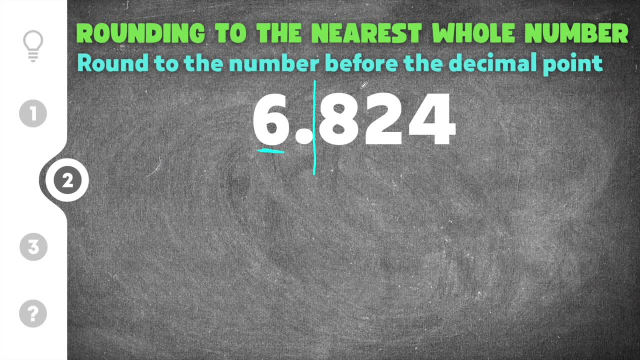 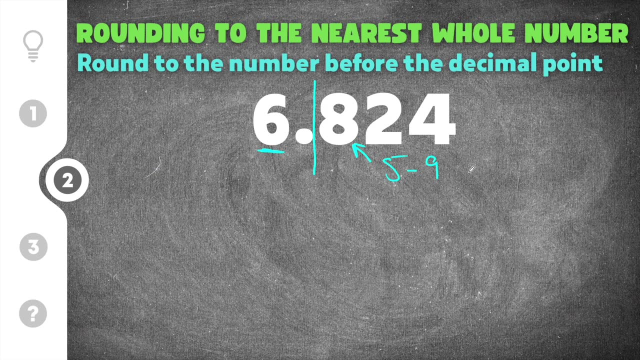 same. In order to determine that, I look at just the number behind my line. In this case, the number is an 8.. Now, an 8 is in between 5 and 9. Which means that I'm going to round up. 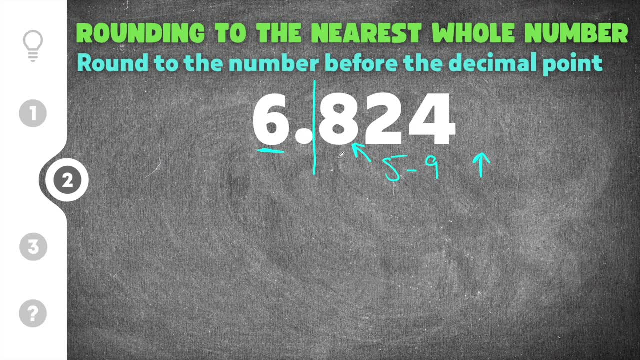 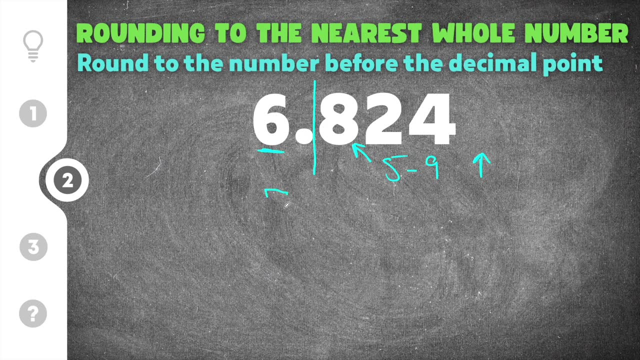 So this 6 is going to get rounded up into a 7, because this 8 is in between 5 and 9.. So it's closer to 7.. So I'm going to round the 6 up to a 7, so I'm going to write 7 here. 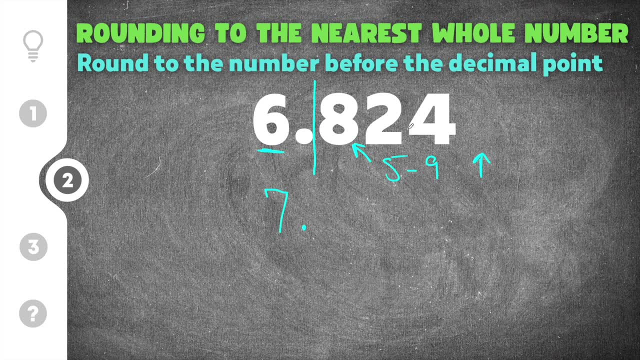 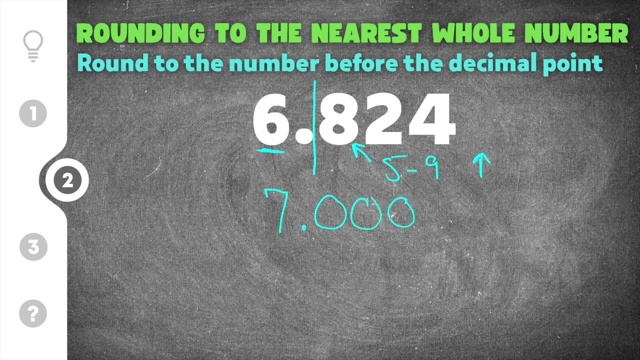 I'm going to put my decimal point right here, and then every number, every digit after that decimal point turns to zero, because we're rounding to the whole number. Now I don't need the zeros because they represent nothing, so I'm just going to write the number.